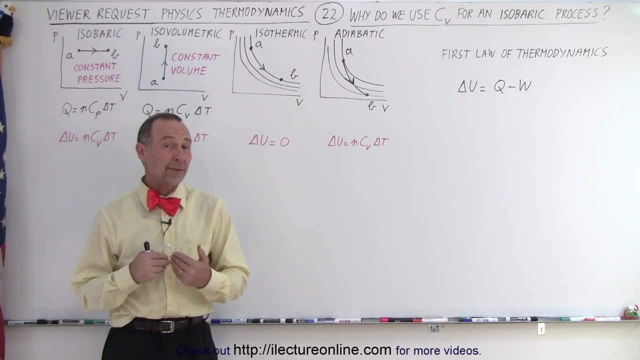 Welcome to iLectra Online. When it comes to thermodynamics, there are two questions we get asked a lot. One of them is: why do we use C sub V for an isobaric process? The other one, well, we'll show you that one on the next video, But let's go back to this one right here. Why is that really a question? 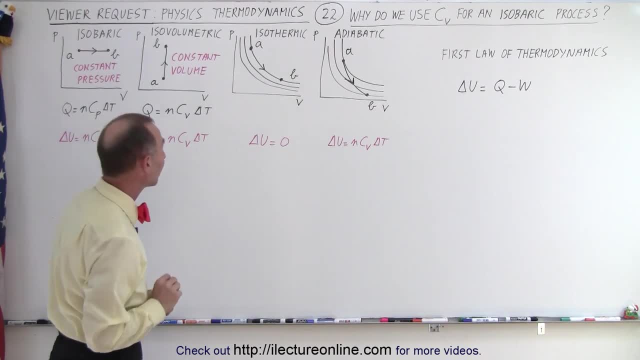 What does that really mean? Well, we have four thermodynamic processes. We have isobaric processes: isovolumetric, isothermic and adiabatic. When it comes to an isobaric process, notice, we have a constant pressure. For isovolumetric process, we have a constant volume, And for isothermic, 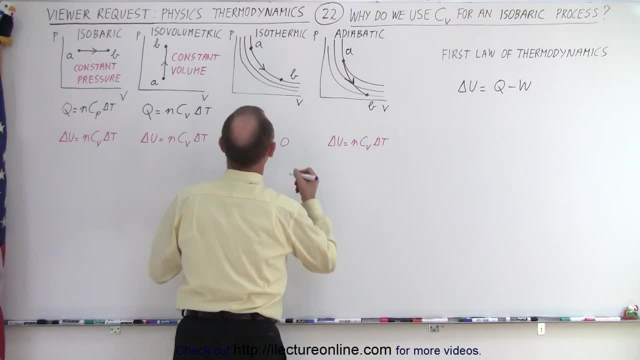 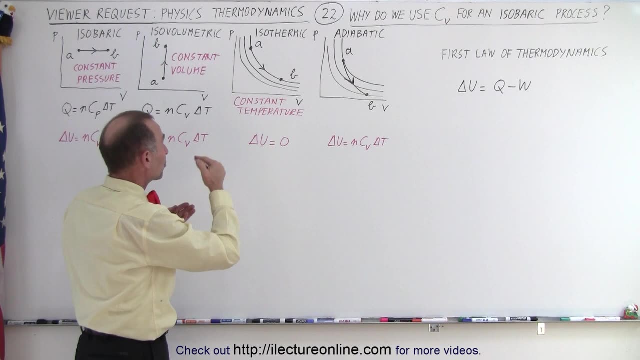 process and I did not write that down. we have constant temperature And also notice. we have the first law of thermodynamics that relates pressure, volume and temperature to one another in any one of these processes. Now the first law of thermodynamics is calledornimagnetic- The first law of thermodynamics. 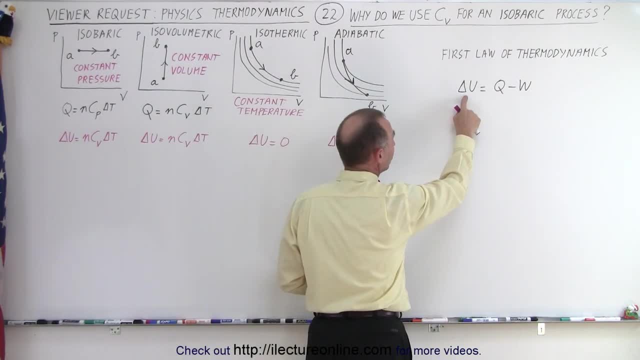 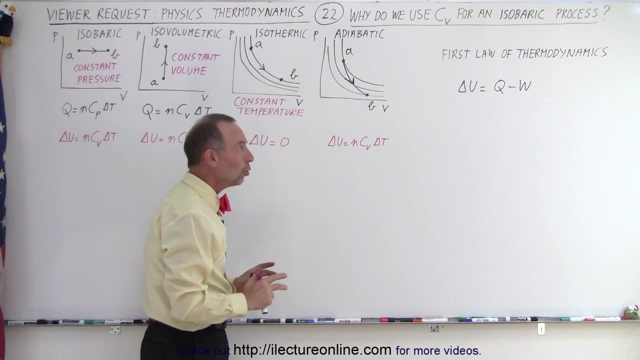 thermodynamics tells us that the change in internal energy is equal to the heat added to the gas, minus the work done by the gas. and so when we try to calculate q- the heat added to the gas or the heat taken away from the gas, depending upon if q is positive or negative- well, it can be calculated. 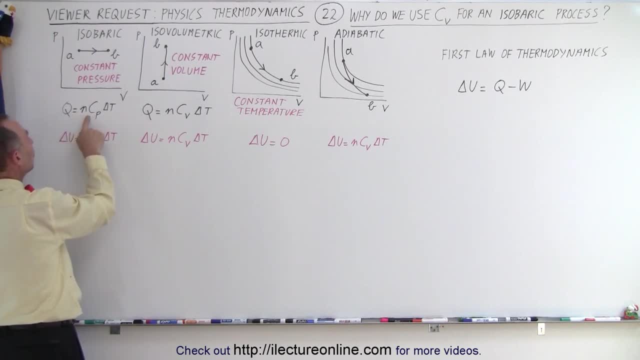 like this, where, where we have q equals n c sub p delta t, when we deal with a constant pressure process- isobaric- and q equals n? c sub v delta t when we try to calculate q- for now it's a volumetric process where the volume remains constant, and so it seems to be clear we use 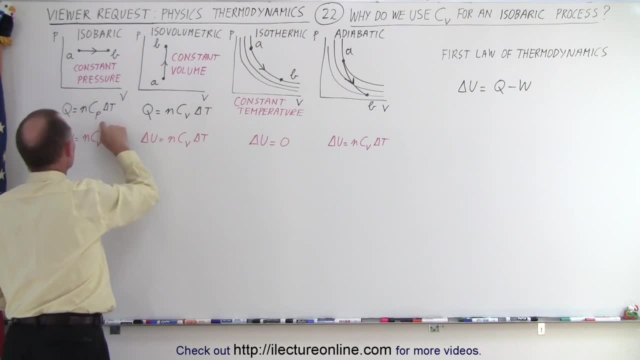 c sub v for constant volume and c sub p for constant pressure. but then sometimes they see me use c sub v in an iso volumetric process- no, not in a isobaric process- and they go. well, i'm confused. why is that happening? well, it turns out it's a volumetric process, so it's a constant pressure. 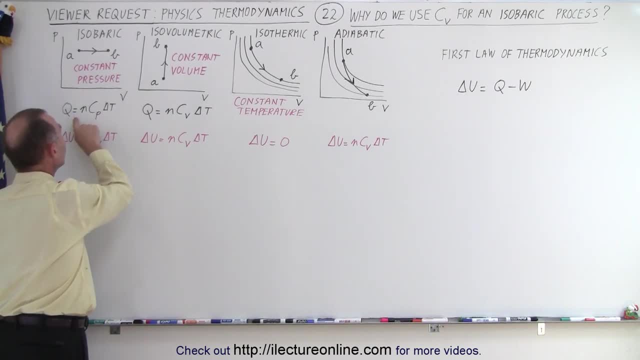 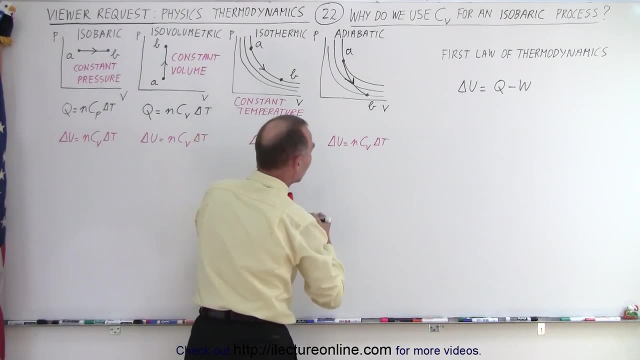 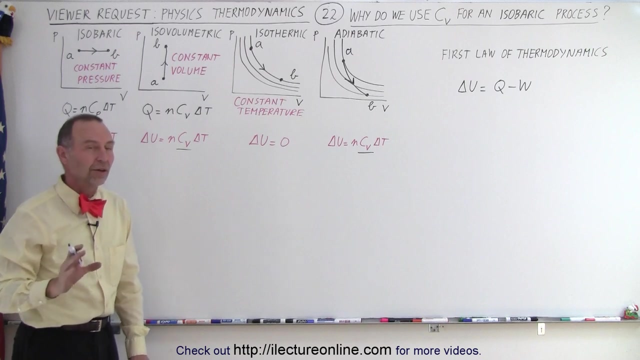 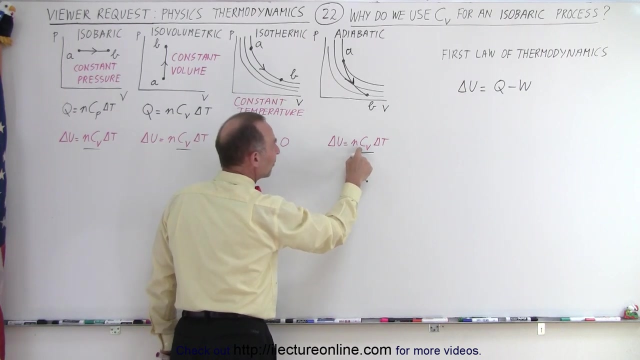 out. we do not use c sub v to calculate q, but when it comes to calculating the change in internal energy, we always use and notice. we always use c sub v, c sub v, c sub v. no matter what process it is, the change in turn in the internal energy is always the number moles times the specific heat. 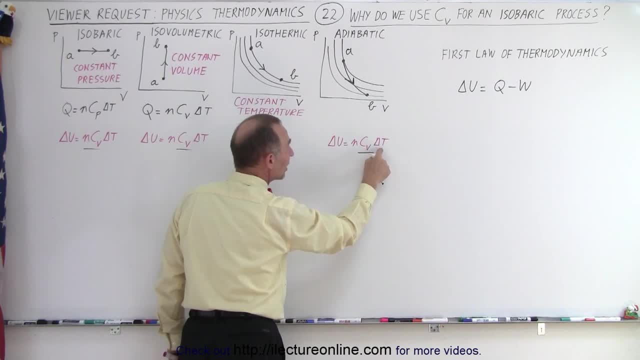 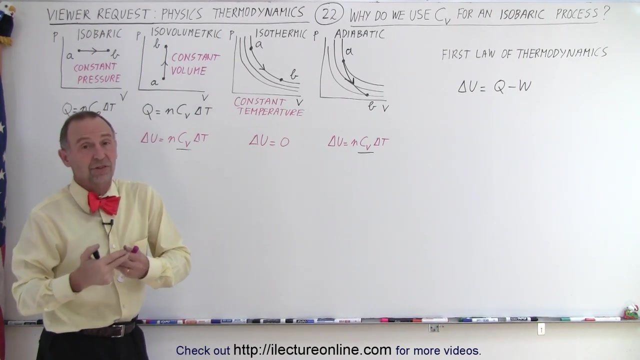 relative to the constant volume times delta t, no matter what process it is, and, of course, for a constant temperature a process, since delta t is equal to zero, delta u is equal to zero. in other words, when we have a constant temperature process, the internal energy cannot change, because the temperature doesn't change. you can only have a. 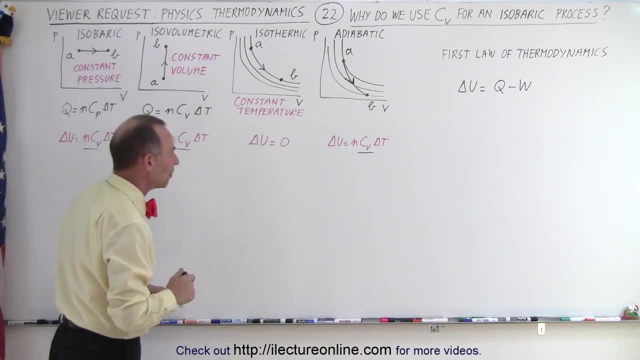 change in internal energy if the temperature changes. so therefore, that is what confuses the students when they look at a thermodynamic process: where does the c sub v come from? well, we always use it, no matter what the process is, and of course here we would use it as well, except delta t is equal to zero. but whenever we're 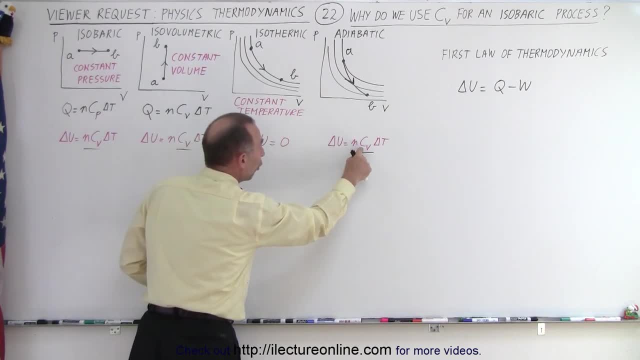 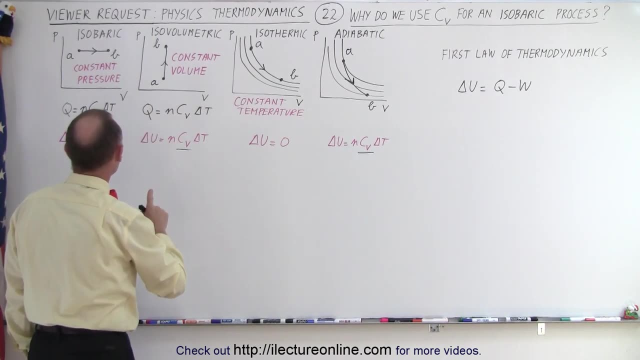 calculating the change in internal energy, we always use c sub v, no matter what process we're dealing with. but when we're trying to calculate the change, the heat added or the heat taken away from a process, then we use c sub p for a constant pressure process and c sub v for a constant volume. 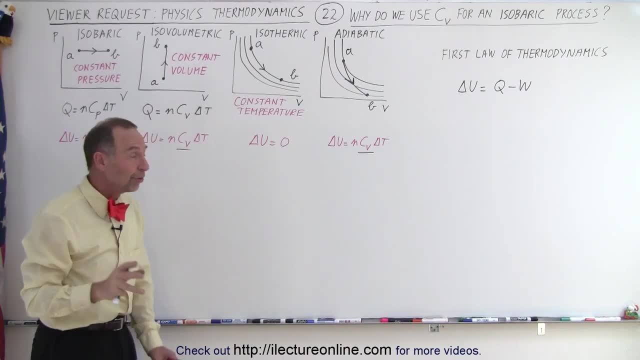 process, and so that is what confuses students. so hopefully, with this video, you'll be able to understand what we're trying to do with this video and answer that question from our viewers. we have it all straightened out and that is how it's done when it comes to thermodynamics. 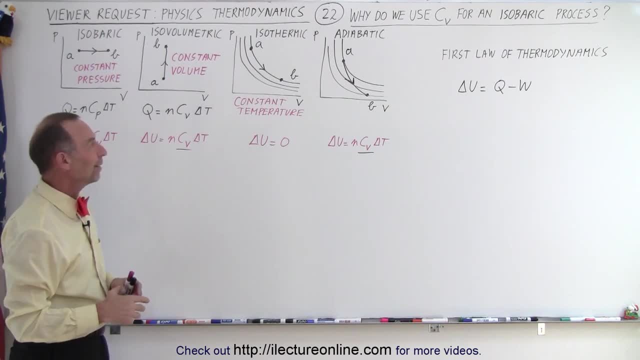 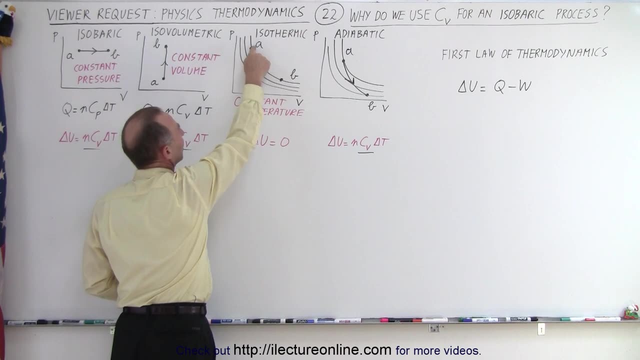 the a to b thing. does that have any sort of meaning? well, yes, the a to b. we use one to two or a to b. it's a process. we start at a and we go to b, so the gas is in this state and then it goes to this state. 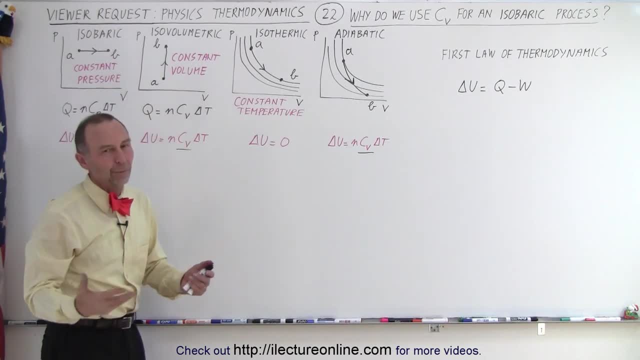 the gas is in this state and it goes to that state. it's in this state, it goes to that state. so that's represents you go from one state to another state, from a to b or from one to two. does that have to be a certain state or any state? it can be any state, but how it changes depends upon which process. 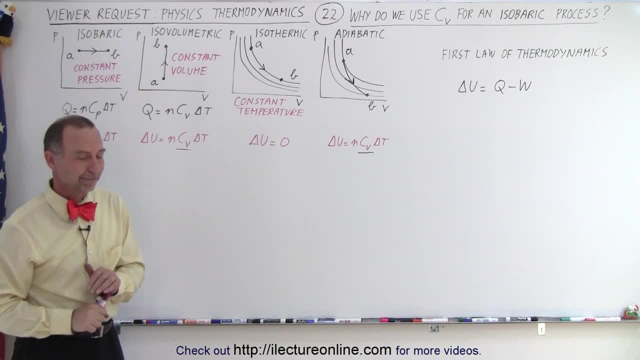 we're dealing with. yeah, okay.